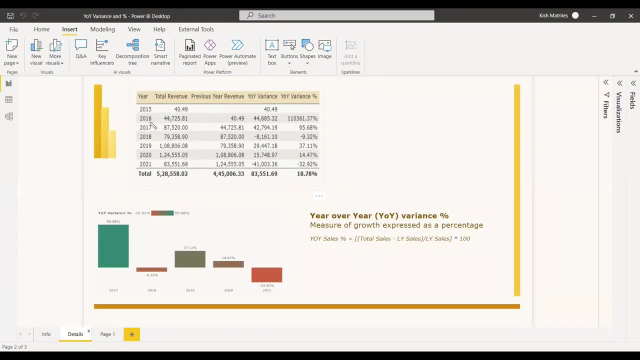 one, So 2000,. you can just take out this 2015.. So from 2016,- if you start by taking 2017, previous year's revenue will be 44,725.. And that will be shown in this tape, column 44,725.. 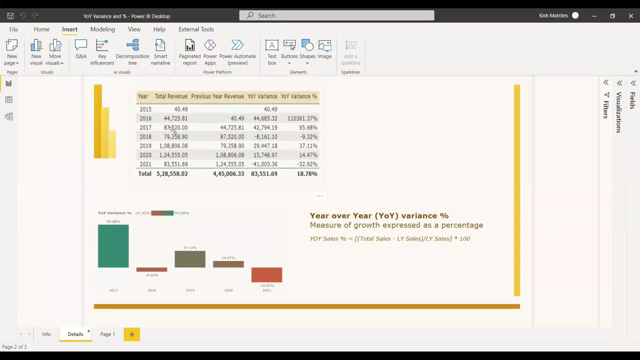 So to get the YOY variance, you need to take the difference between this total revenue. That means the current revenue of 2017.. And you need to take the difference with the revenue of 2016.. That is 44,725.. So you will be getting a result of 42,794.. This is the YOY variance. So if you 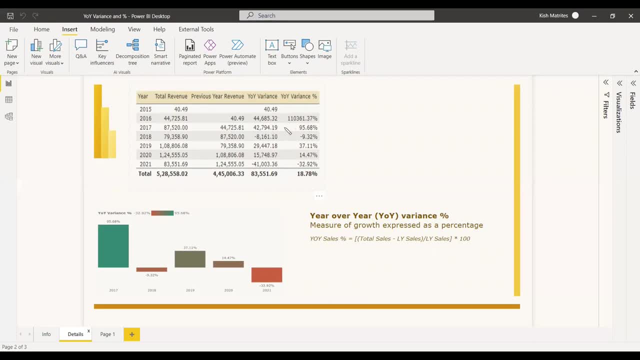 need to get the percentage of YOY variance. you need to divide this YOY variance with the previous year, which is 44,725.. So you need to do it with respect to all the years. then you will be able to understand the measure of growth in these years for your company or for your product. So that is. 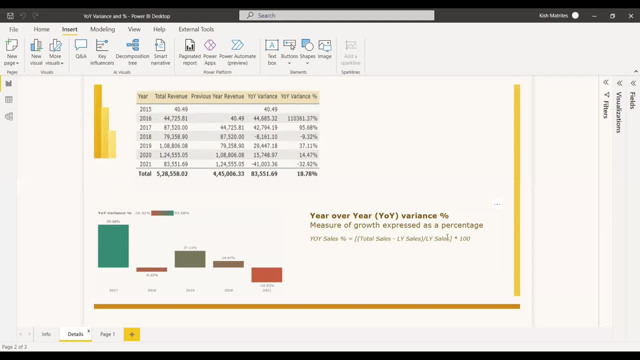 the definition itself of where you can measure the growth expressed as a percentage, So the percentage. you can understand, okay, how well your growth is going along with the years. So you can see here, since it is a first year, it is having a good growth of 95%. But in the second, 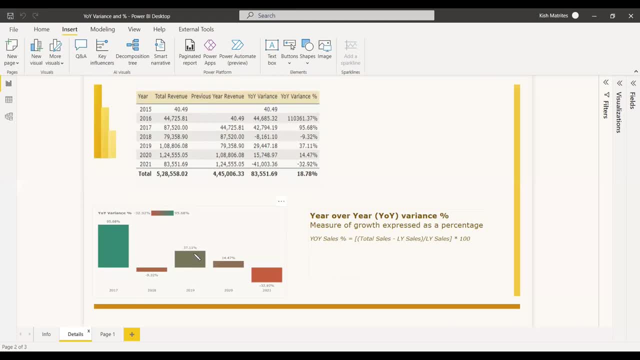 year it went down by 9%. The third year, of course, it got back 37. But in the fifth year, that is, 2021, it went 32% down. So you can plot it in a chart also And you will be able to. 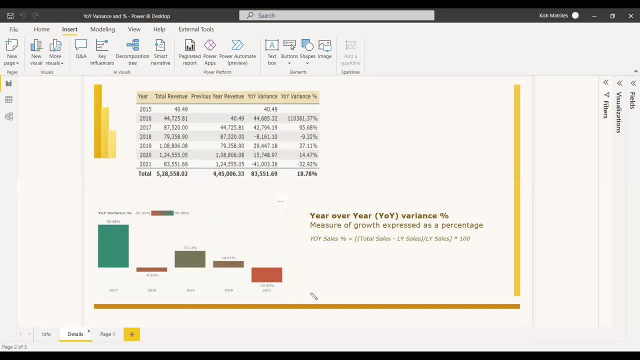 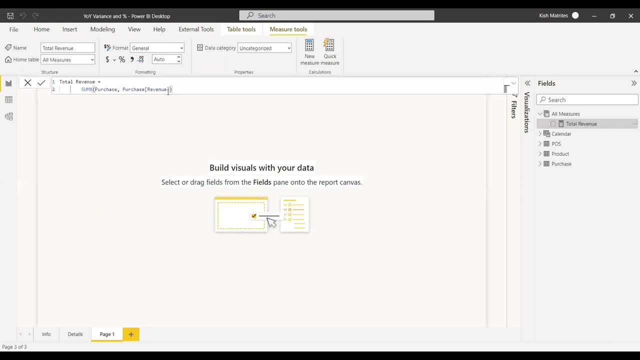 understand that through this visual, how the measure of growth is going along with the year. We will be doing the same example. We are having the data set, we are having the total revenue, that is the sum of revenue, and we will be having a calendar And in the calendar, 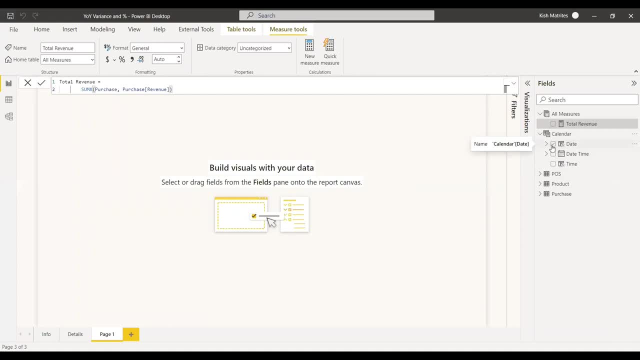 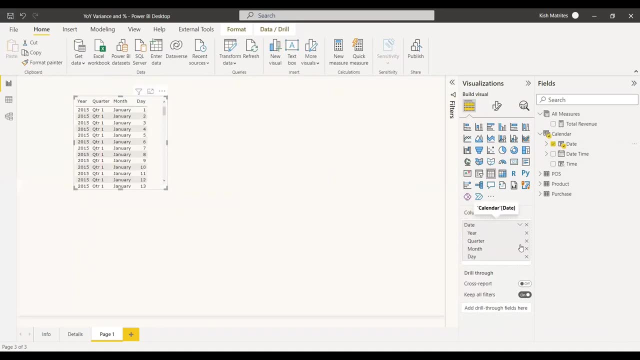 we are having the date column where we are having the hierarchy of year, month and date with quarter. We will take a table visual And in this table visual we will get the year, all the years we will take, and we will get the total revenue of the years Now we will create. 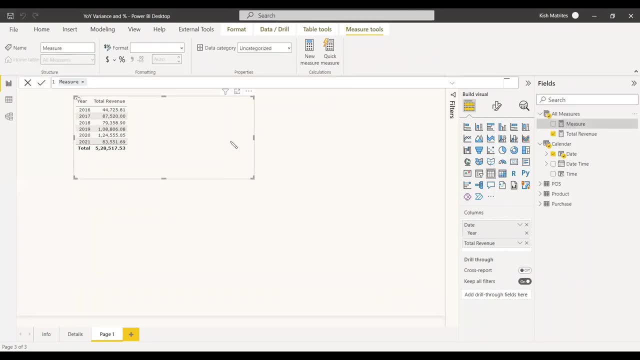 a measure for previous year. So for getting the previous year you can use the DAX function and date add. With the date add function you can get the previous year revenue, So we will write it as previous year revenue. It goes to calculate total revenue And from this total revenue. 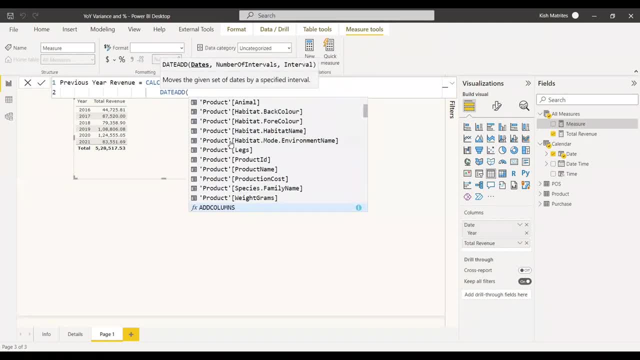 you can filter it by previous year So you can use date add function and calendar. date And number of interval is just last year, so minus one, And the interval you need to give it as year since we are getting the year, So you can drag it That also inside First year's difference. 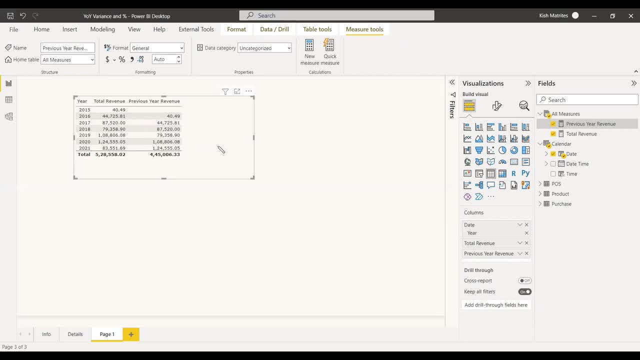 44,725,. it will be a huge margin. So we can avoid that in the graph because of course this is the start of year, So definitely you will be having a big hike. Now we need to get the difference between these two columns, That is, the current year's revenue and the previous year. 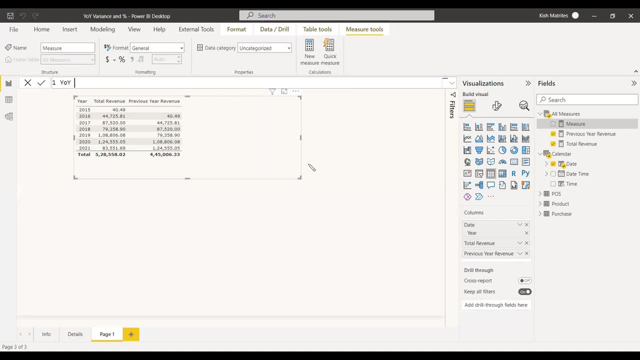 So you can create a measure for that And name it as YOY variance. So the difference is called variance. So you can take the total revenue, That is a current year's revenue minus previous year's revenue, And you can select that inside the table And of course the first year it will be 40. The 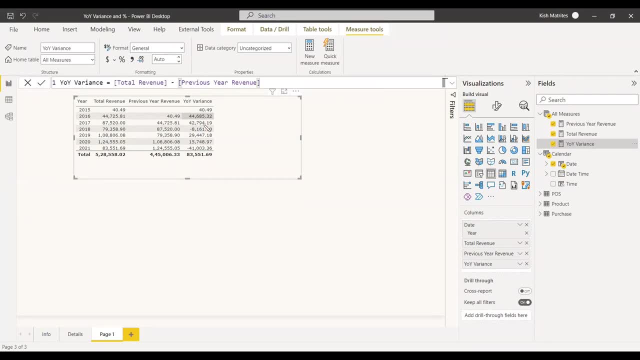 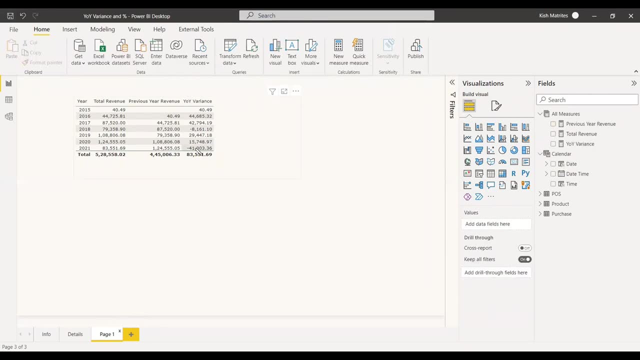 second year it will be a huge margin. Third year also there is a huge margin. Fourth year onwards we can understand the exact growth We can understand from the fourth year onwards. So the fourth year it has gone down, Then it has come up Once again. it has come up a little bit. 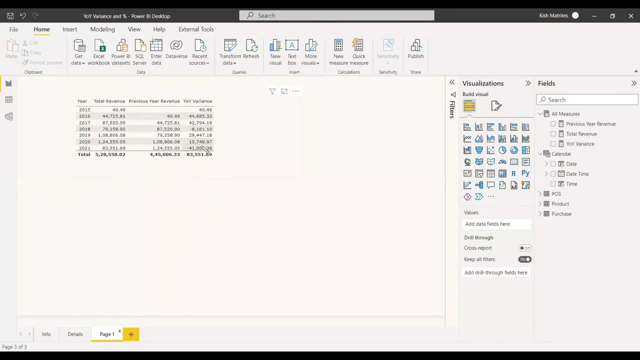 Then it is going down a huge margin. So in this way you can understand the variance. But if you get the percentage, it will be more easy how much percentage you can understand. So it will be more clear. The growth rate will be shown very nicely, So you can create a measure for that. So 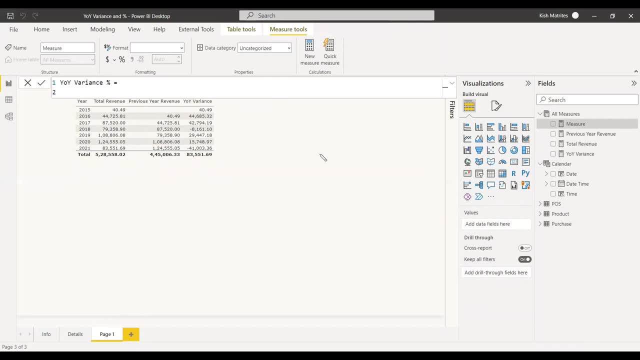 you can see that the YOY variance percentage equals to: We can just divide the YOY variance with the previous years. Now we need to select this And you can select the percentage. Since this is percentage, you need to select the percentage symbol here, And now we can select the. 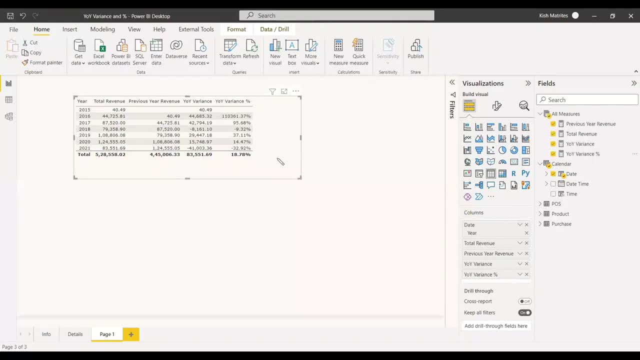 YOY variance percentage inside the table. So here we can understand that the first one is this much percentage because from 40 it is on to 44,000. But the other one you can see minus 9,, 37,, 14,, minus 32 percentage It is. 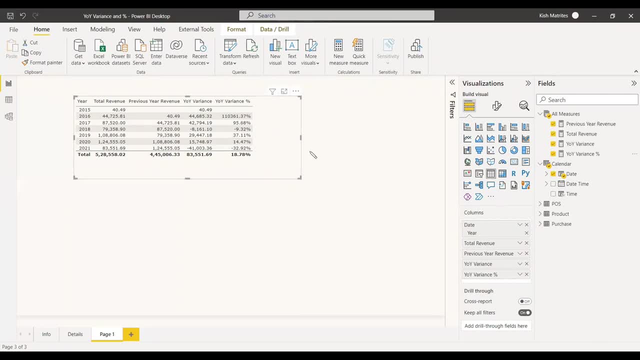 going down and it is fluctuating like going up and down. Through this way you can understand the growth and the level, how the company is moving forward. So you can use a cluster chart, Visualize this So it will be more useful for the end user to understand it more clearly. You can select the 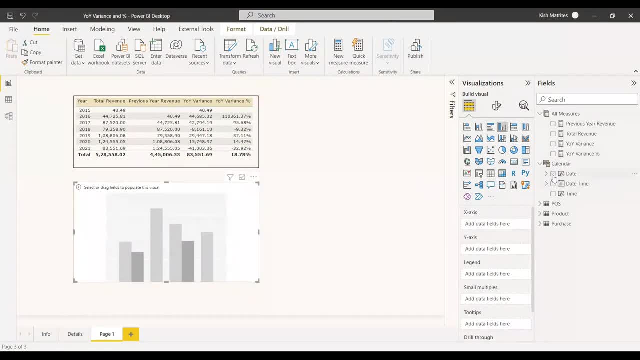 cluster chart And here in this cluster chart you can select the date And from the date you can select the year and remove all the other quarter, month and date. Now you can just select the year YOY variance, And here we are not able to see any other. 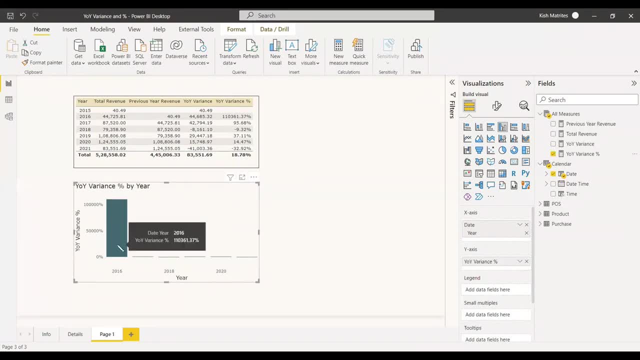 columns because the first column is showing too much. You can just right click here and exclude the first column. It is like almost like filtering it out. So when you go to the filter here and see that it has been filtered out, So we are getting the values from 2017 onwards Actually. 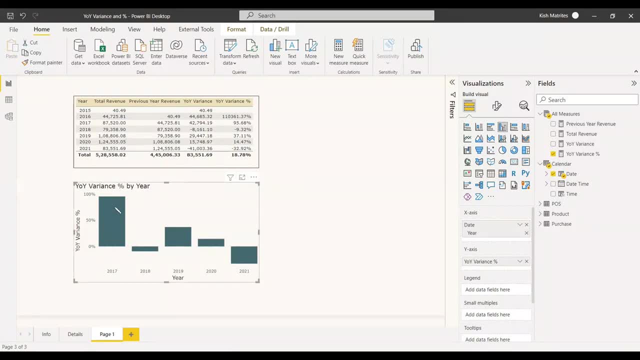 from 2018, it is going in a smooth. Only for 2017, it is in a very higher rate. The remaining it is going smoothly, like just fluctuating, fluctuating a little bit: 30%, 30% here and there, So you can. 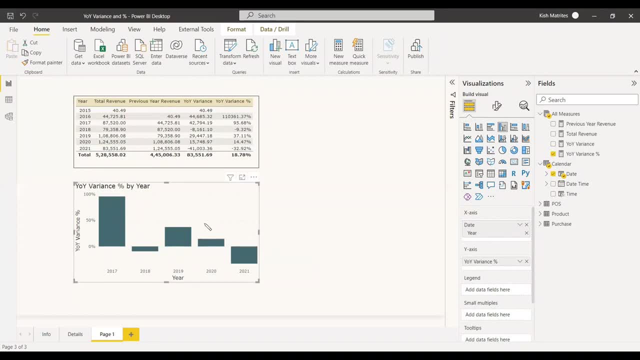 visualize it more clearly by using a cluster chart. So you can visualize it more clearly by using a conditional formatting to these columns. You can go to the visual and you can go to, of course, you can give the data label And then you need to go to the columns And in these columns, the column 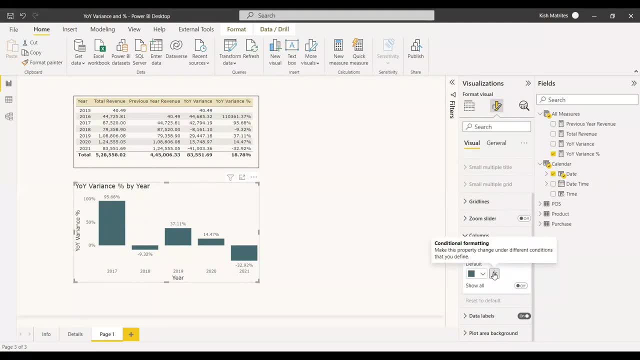 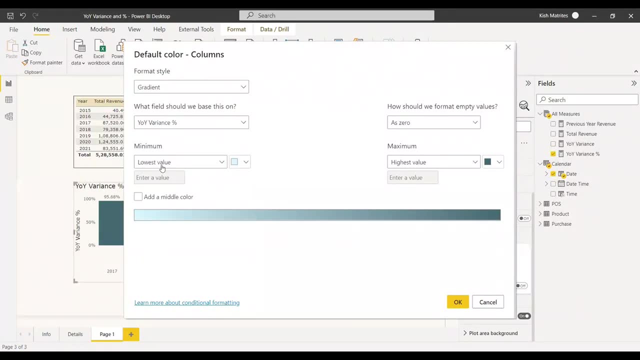 default color will be shown here. You can go to the function conditional formatting And in this function which field you need to format. you need to format the variance So you can get the variance here, The lowest value. you can give very, very light or thin color And of course it has already. 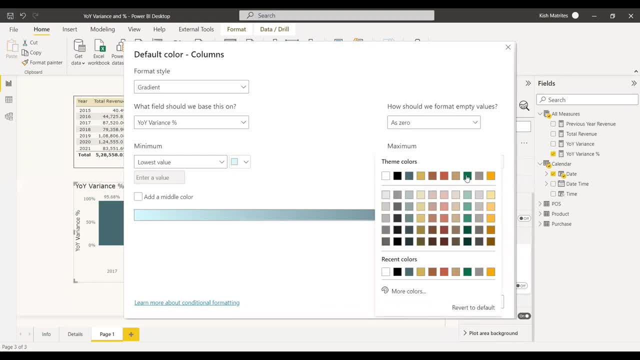 given And the highest value you can give the dark color. So usually you can give here green, give your red color. Red color should be given more importance because when you show the red color, the end user will understand: okay, you need to give more importance to these. 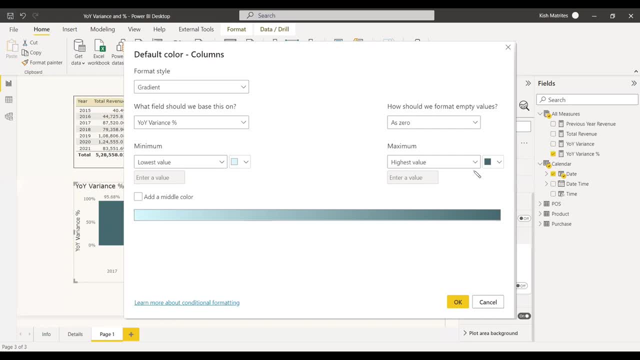 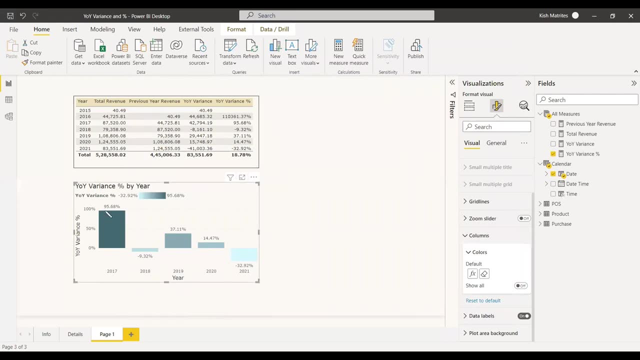 red color values. So here itself we have given very low color, light color, and we have given the hard color here for the maximum value And we will see how it is. So you can understand. okay, the hard color, that is the growth, that is 95%, is just showing very thick in color. 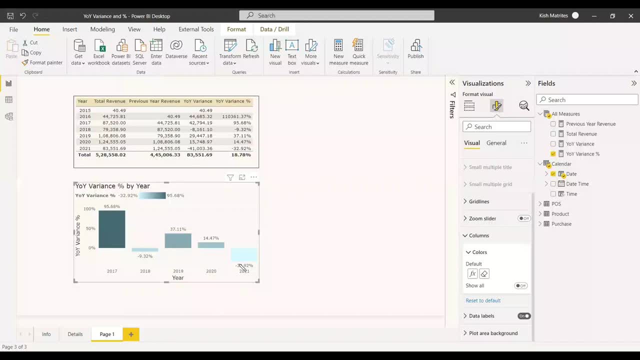 And the growth which went down. that is showing light color. And this growth has gone down 32%. It is showing very, very light color. If you want to change the color and reset to the default, you can just wipe away the color by just clicking this rubber button. You can give it a red and blue. 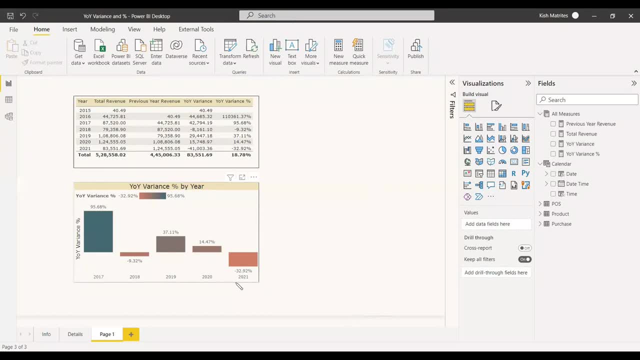 itself. So in this way you can plot the YOY variance percentage using a clustered column chart. So this will be more meaningful when you give a mid value or something and then you can plot it in a very meaningful colored way. So if you want to have a slicer for the products you